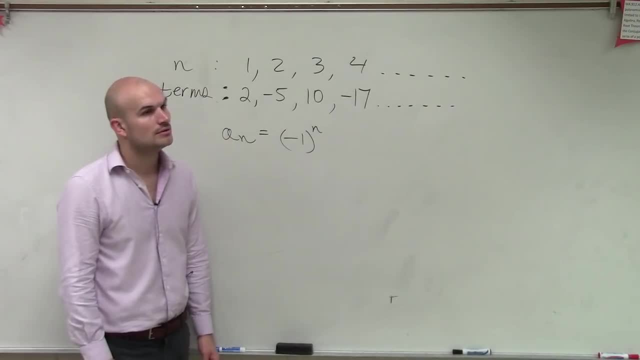 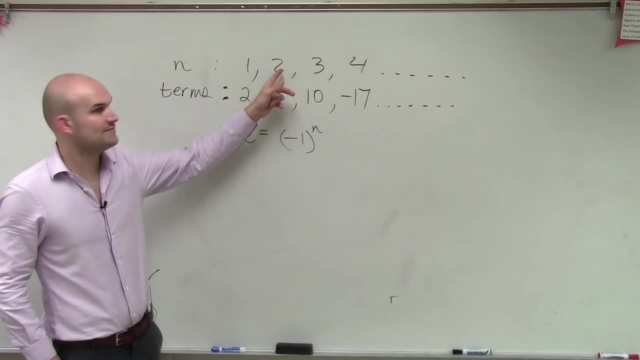 But that's even. It's the second term, so that means it's going to be even. And then to get the negative you have to multiply by a negative 5.. So that's what I'm saying. If you did 2, right, if you multiplied it by negative 2,. 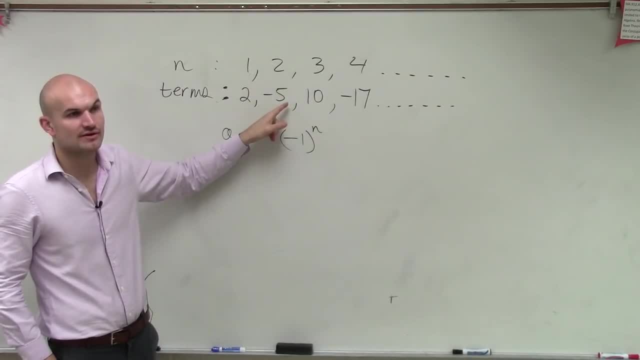 right, and then subtracted it from 1.. Yeah Right, That would give you negative 5.. 2 times negative: 2 minus 1.. Negative 2 is negative 4, and then minus 1 is 5.. All right, Now let's see if that would work for this. 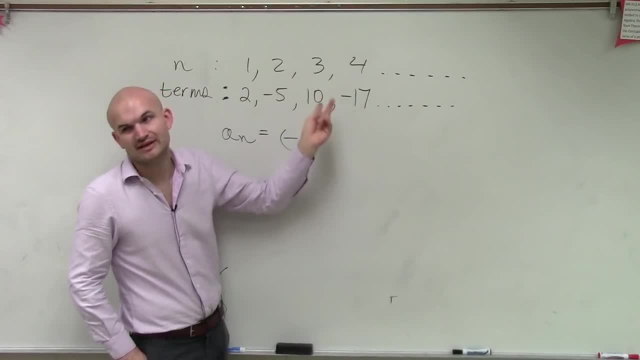 2 times 3 is 6, minus 1 is 7.. Well, that's not even getting me close, right. I'm not worried about the alternate signs, because that's just going to alternate signs, But now I'm not even close to that, right. And then 4 times 2, that's not going to work. 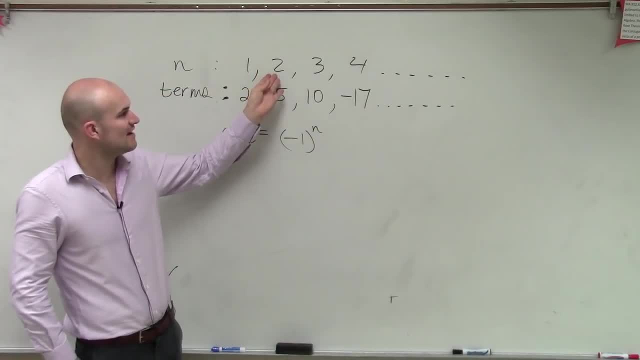 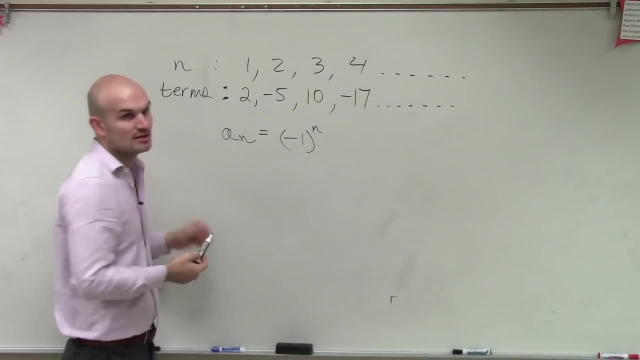 So now I need to think of a different relationship. How can I get from these values? So we kind of marked off adding and subtracting. right, I can't add or subtract my terms. I can't when I plug in 4, I don't know why I was looking at these terms originally. I 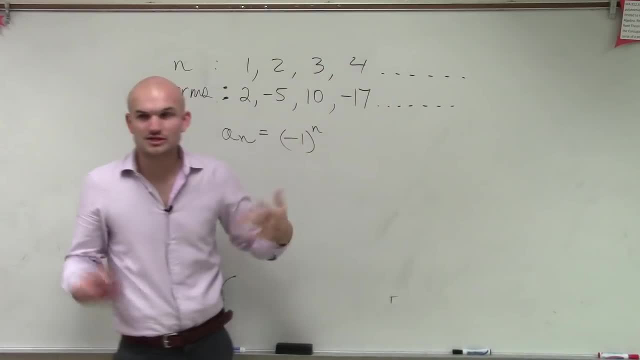 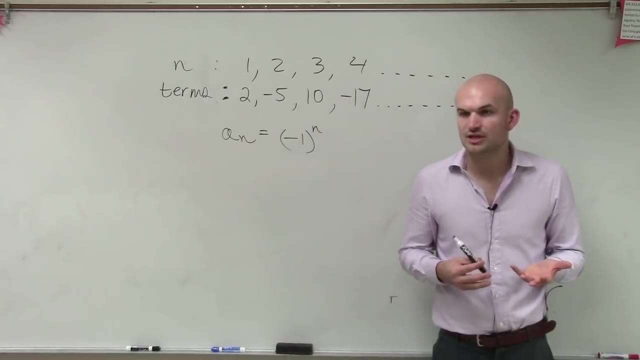 can't add or subtract 3 to get 10, because it's not the same. So there's another relationship: Adding and subtracting are out, Multiplication and dividing are out. What's another way that we could? what's another relationship or another operation? 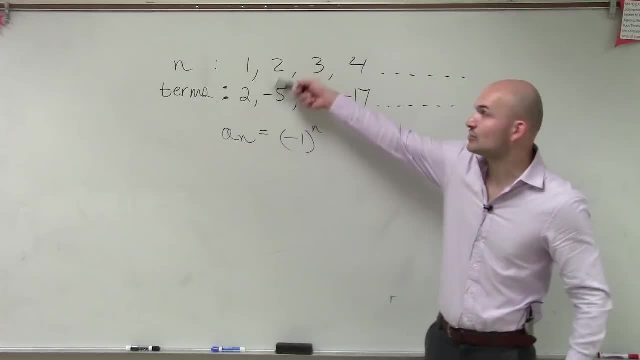 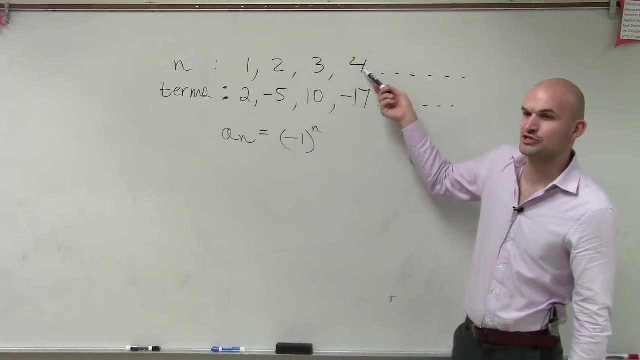 Subtraction. Well, adding and subtracting are out. We can't add or subtract. the same number for each one of these terms Factor. So if I take the square root, but these numbers, if I take the square root of 4, that's: 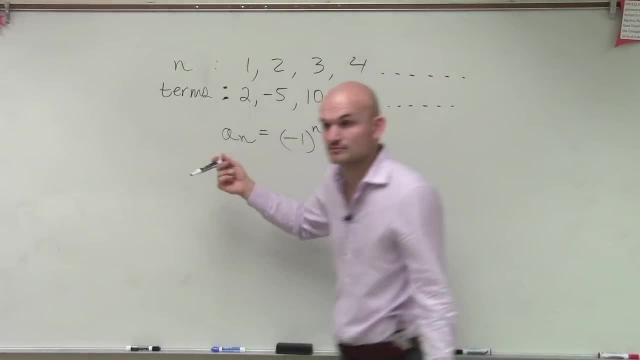 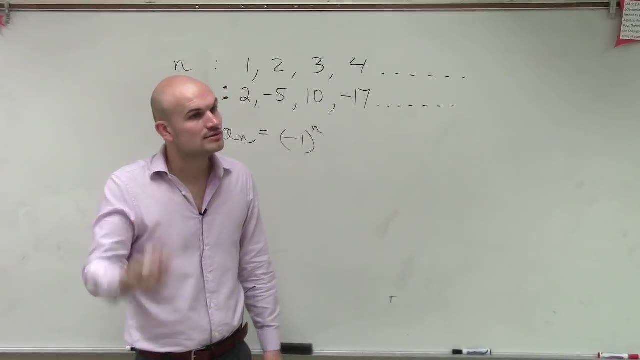 2, that's not close to 17.. But what's the opposite of square root, Opposite of square root? Squaring, Squaring. So let's see if squaring does that get us anywhere close. If I took 3 and 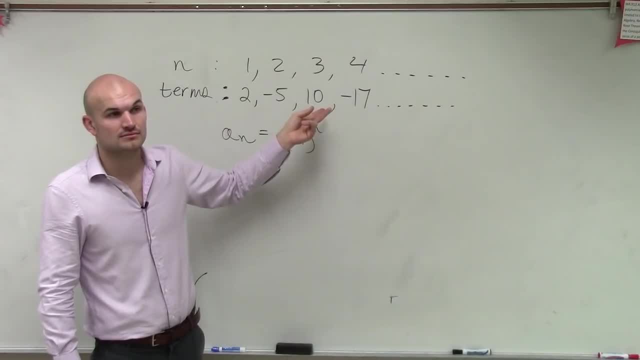 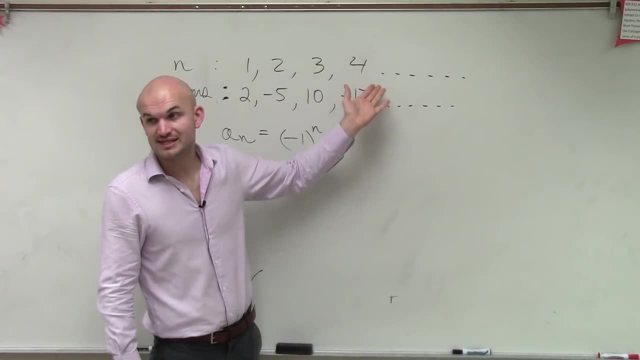 squared it, that's 9,. what would I have to go to get to 10? Add 1, right? Would that get me close here? If I did 4 times uhm, 4 squared would be 16?. 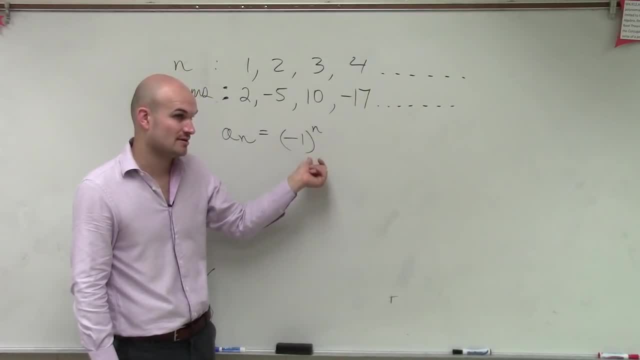 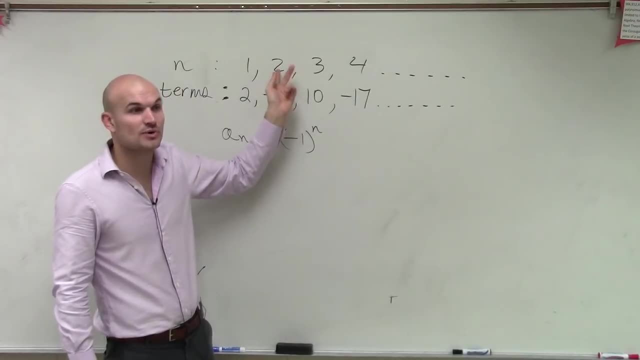 be 17. it is negative, but remember, we have the negative component here, right. but are we getting, I know, but I'm just saying, are we getting close to our numbers? 2 to 2 squared plus 1 is 5, right, so that's something good. so we have n. 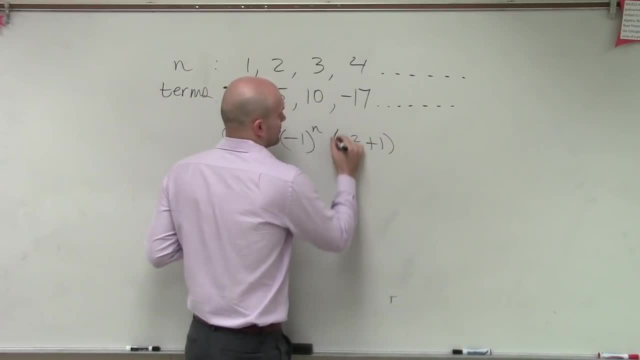 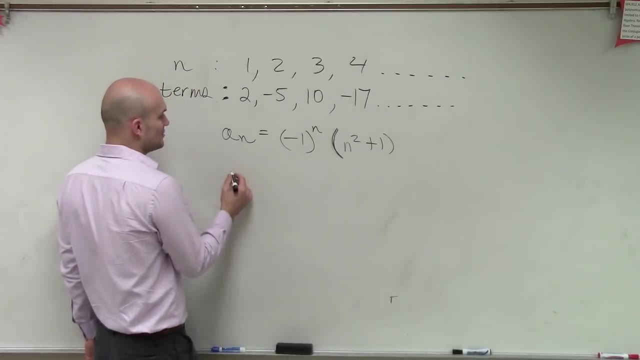 squared plus 1. now we just need to make sure. how is this going to work? all right, so let's see, does this formula work? let's do a sub 1. a sub 1 equals negative 1 to the first power times, 1 squared plus 1. well, negative 1 squared is: 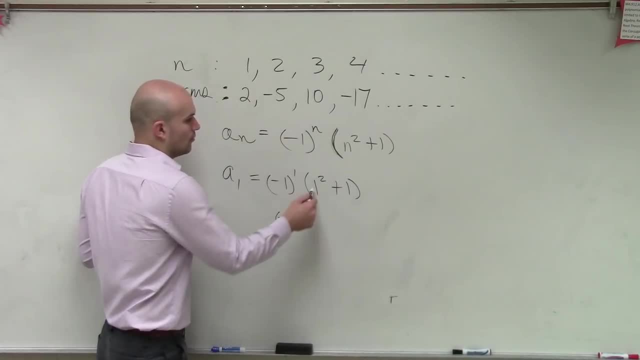 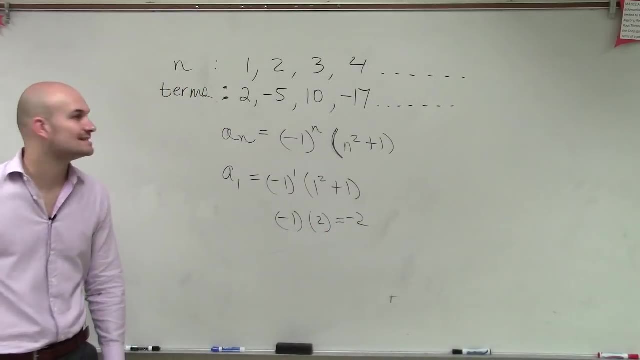 negative 1. 1 squared is 1 plus 1 is 2, so that equals a negative 2. we need a 2 right, not a negative 2. so I'm close, but I have the wrong sign. so something I need to do to maybe change this. 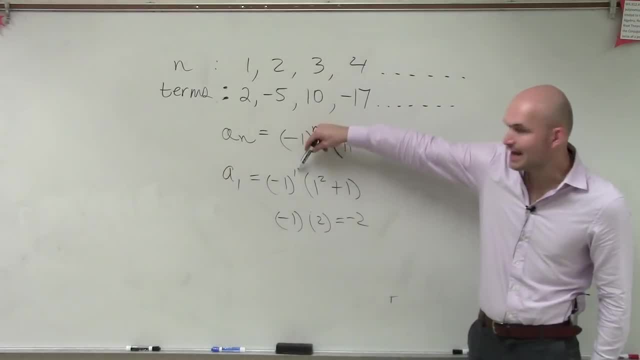 so maybe what I could do is so, since this is starting off a negative, that means I'm starting as an even, as a odd power, so I probably want to start this as a even power. so what could I rewrite? instead of n, I could write it as n. how? 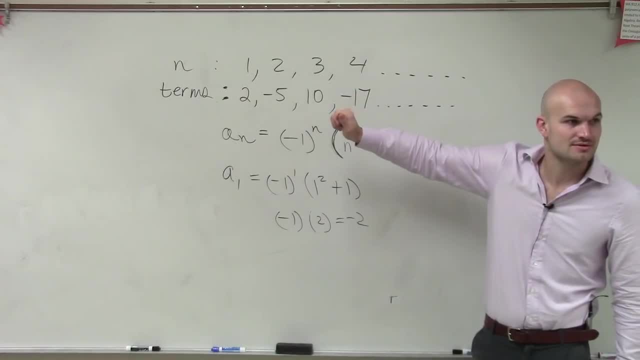 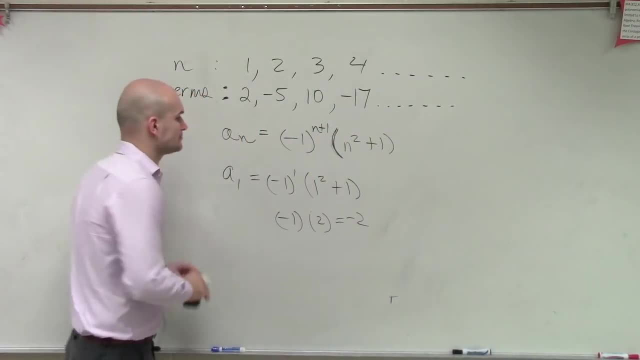 could I make an odd to an even? I just have to add how many values one. so let's try this: n plus 1. so now let's do a sub 1 negative 1 times 1 plus 1 times 1 squared plus 1. 1 plus 1 is 2 negative, 1 squared is or: 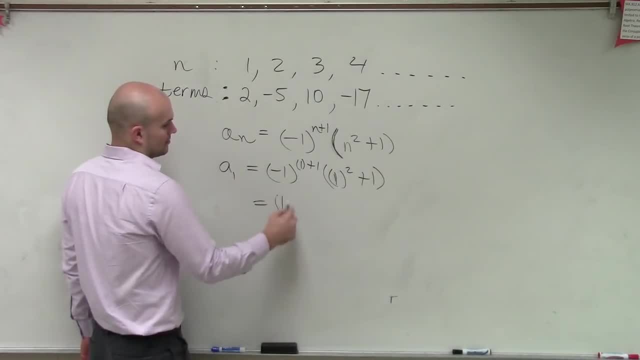 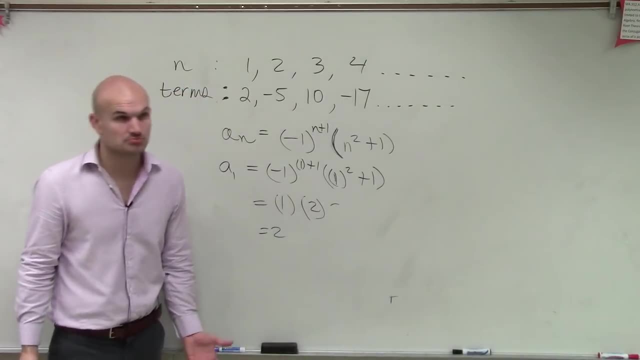 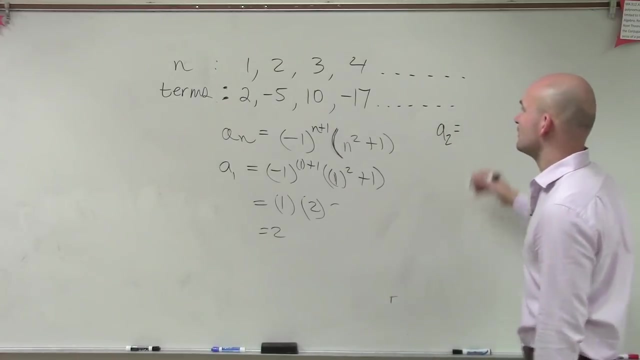 negative: 1 squared is 1 times 1. squared is 1 plus 1 is 2. looks pretty good, right? let's try another one, just make sure our works correct. let's do a sub 2, so if I I do ace of 2, I have negative 1, 2 plus 1 times 2 squared plus 1.. 2 plus 1 is 3.. Negative: 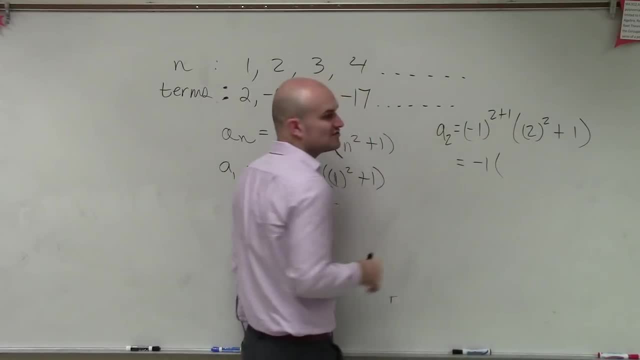 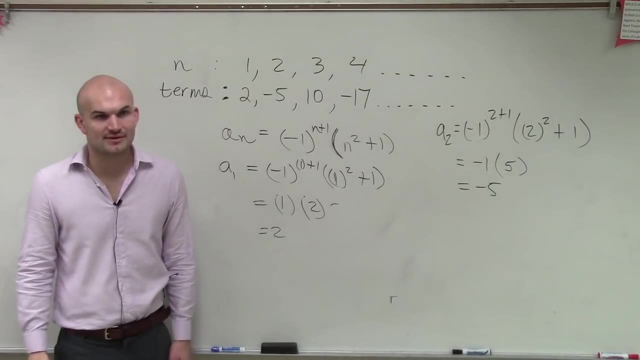 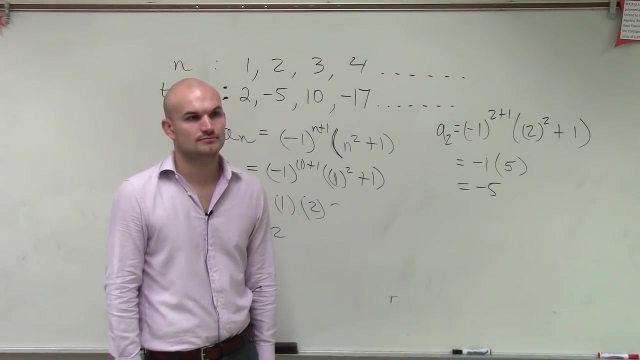 1 cubed is negative: 1.. 2 squared is 4 plus 1 is 5.. Are we thinking like we're on the right path? Yes, Okay, Yes, Yes, We're not really guessing, We're just kind of working. 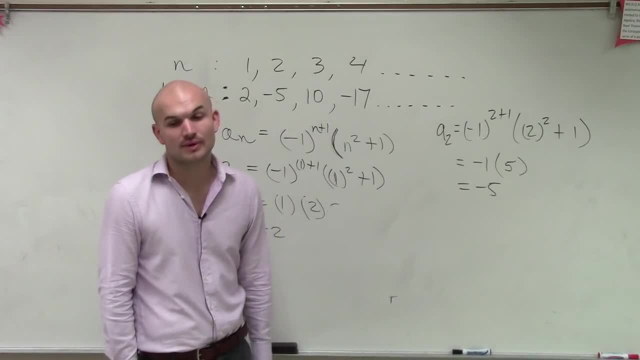 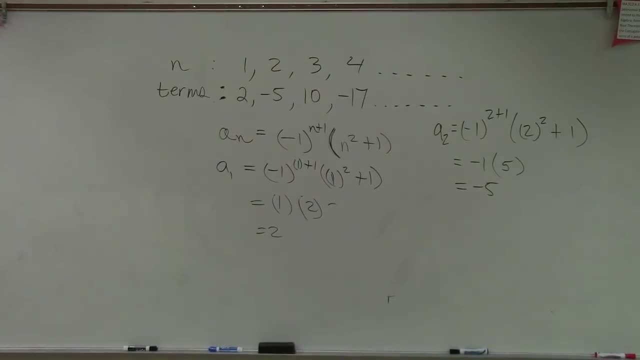 through what the relationship is. We're going through there- And, yes, that's what. that's exactly what I was trying to describe to you guys is, ladies and gentlemen, the first thing we learned.